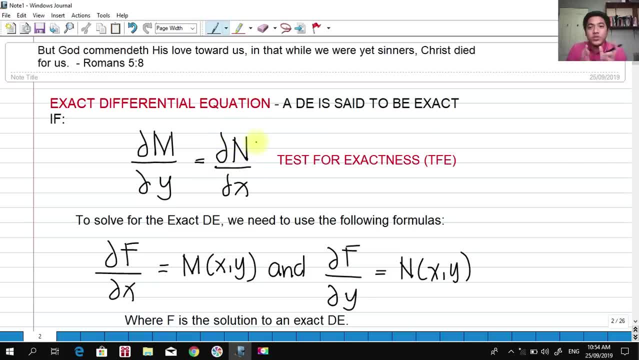 And the N term is also a function of X and Y that is associated with the DY in our given differential equation And this is also called the test for exactness. If we're going to test for the exactness of a DE, we're going to use this formula. 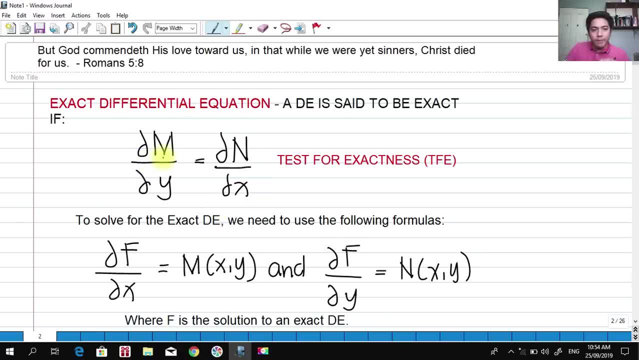 If they are equal, if the partial derivative of M with respect to Y is equal to the partial derivative of N with respect to X, then it means that the DE is said to be exact. Well, of course, if it is not equal, then it is not an exact. 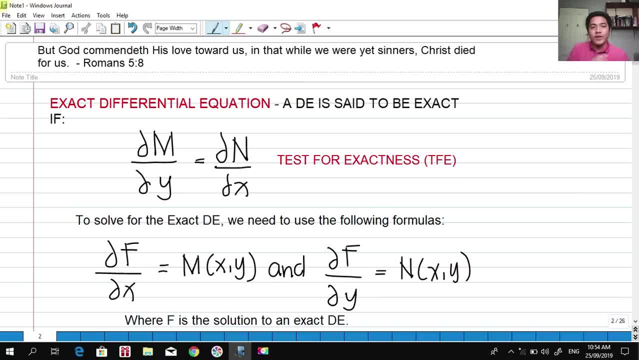 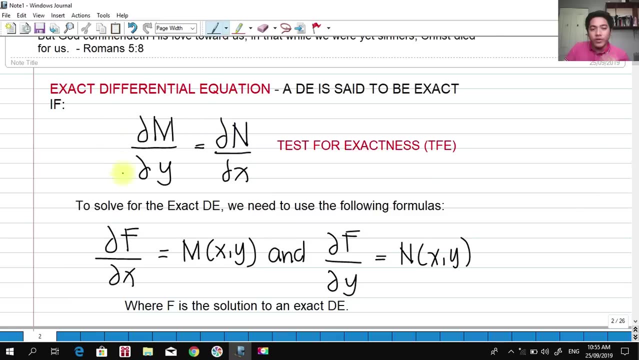 But in this case we're going to talk about or solve problems that are exact differential equation. And if we fulfill this, if we computed this to be equal in our TE, then to solve for the exact DE we must be using these formulas. 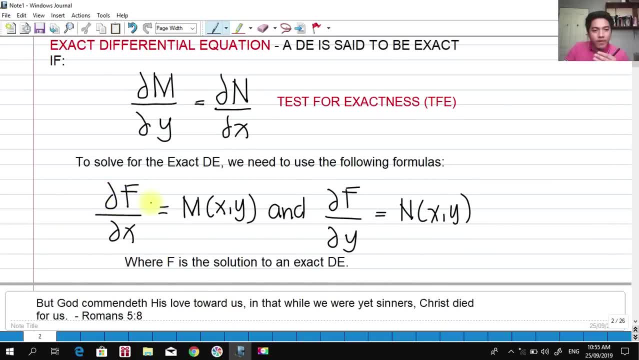 We're in the partial derivative of F with respect to X, And the partial derivative of F with respect to Y is equal to the function of M, M, X and Y, And the partial derivative of F with respect to Y is equal to the function of N, X, 1.. 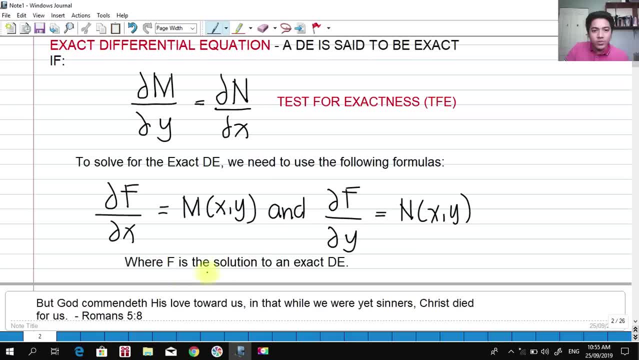 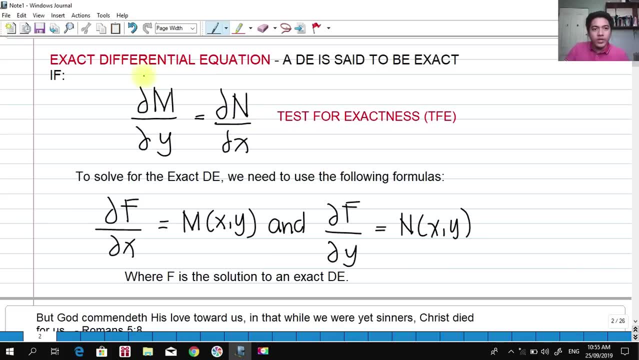 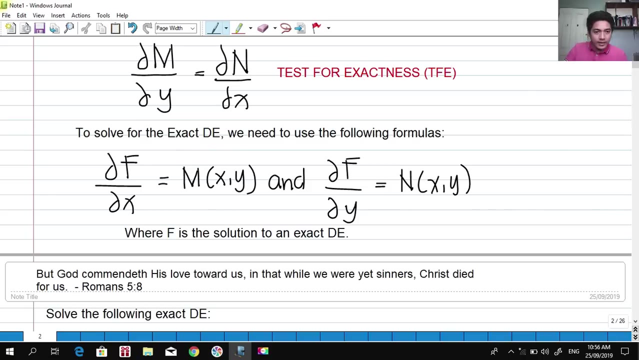 So where F here? where F is the solution to an exact DE. So, in other words, if first, if we are solving exact DE, we need to first test for its exactness. After we test it for its exactness, to be proven that this is an exact DE we're going to solve, we're going to use this formula to solve the exact DE. 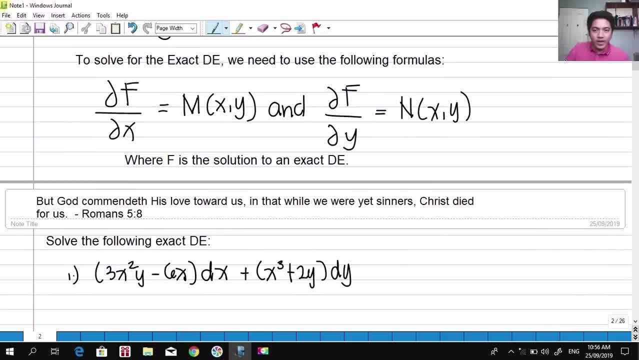 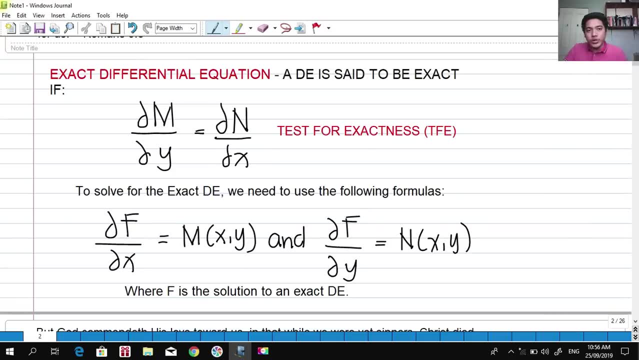 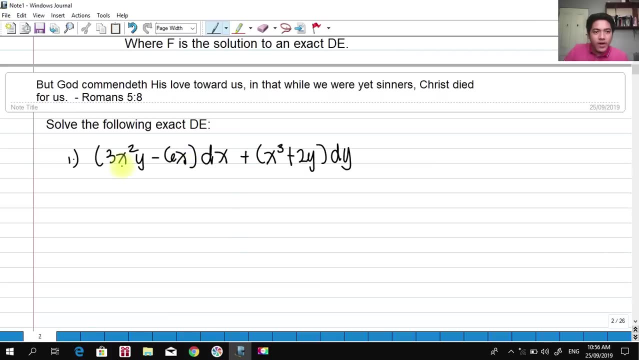 Okay, So let's try to solve this. Okay, So in this exact DE, you will be recalling your knowledge: all about partial differentiation, of course, integrals, Okay, And some of algebra. So let's try this. Solve the following exact DE. 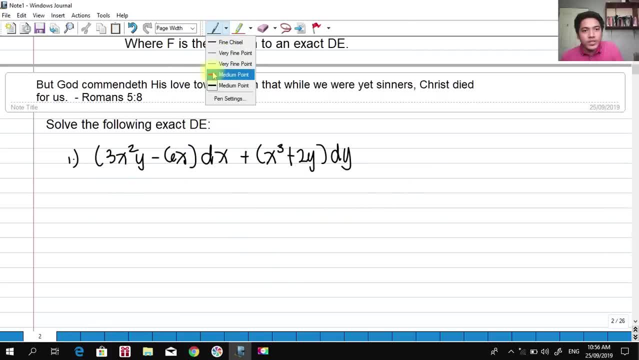 As we all know, again in our previous video we discussed that all the terms containing XY- okay with the DX, that is, our M, and all the terms here with our DY- is equal to N, So this should be equal to 0.. 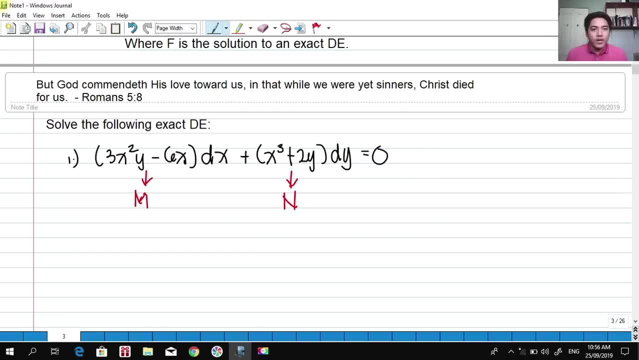 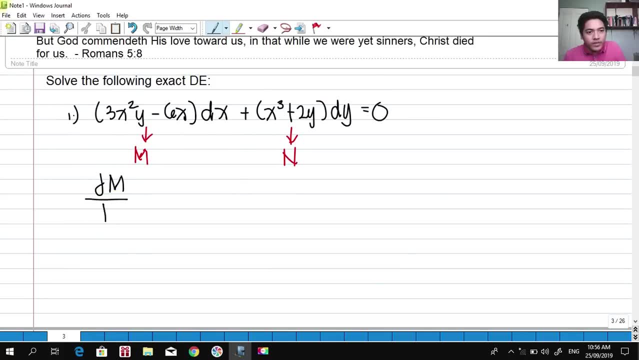 Okay, I forgot to write it. So to solve this class. okay, we're going to test for its exactness. That is the partial derivative. So the partial derivative of Y of M with respect to Y is equal to the partial derivative of N with respect to X. 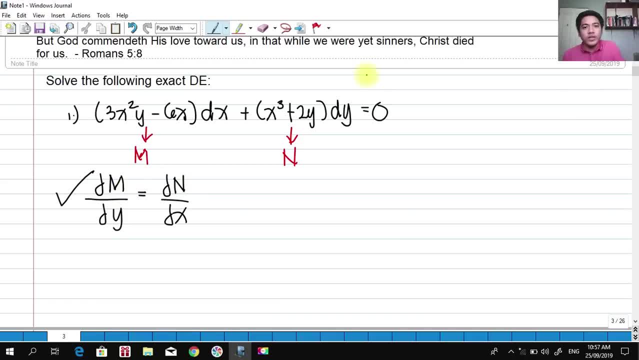 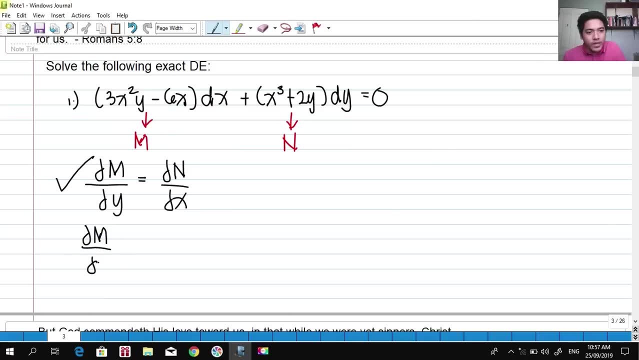 So we must test this in order for this DE to be exact. So, first of all, we're going to get the partial derivative of M with respect to Y, So we're going to get the derivative of this with respect to Y. What is our M? 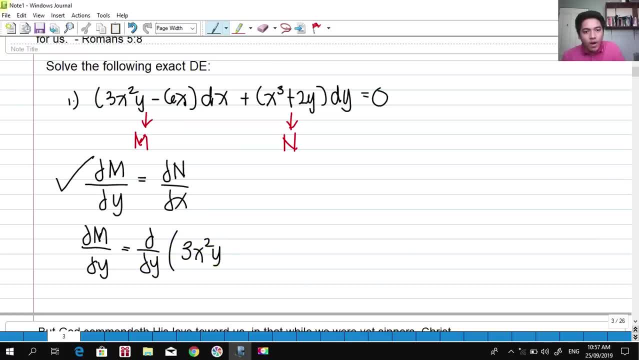 This is our M 3X squared Y minus 16.. That is our M with respect to X. Okay, So take note that this is a partial derivative. So if we get the partial derivative of M with respect to Y, we're going to treat other constants. 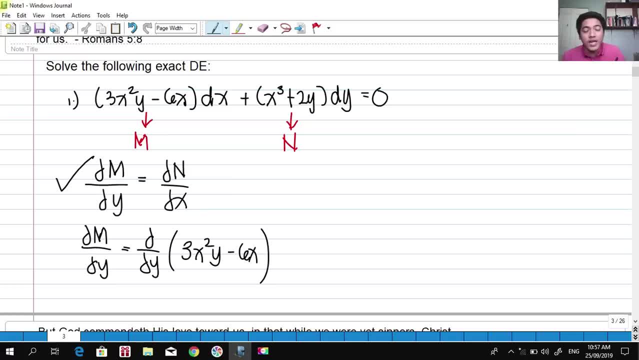 aside from Y, okay, or other variables aside from Y as constant. So again we are differentiating with respect to Y. So all of the other variables other than Y is constant. So in this case We can say that if we get the partial derivative of this M with respect to Y, okay, we will. 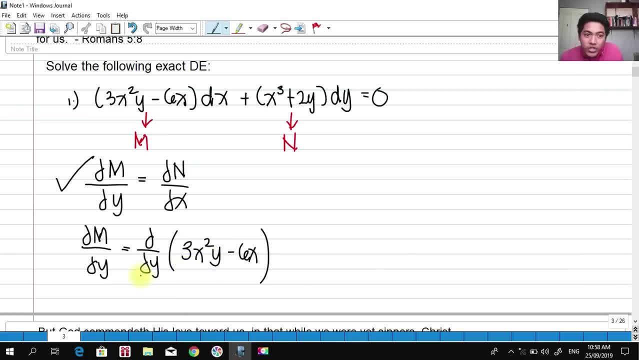 be treating X as constants because we are differentiating with respect to Y. So what will happen here is that 3X squared will be constant. okay, So that is a constant and differentiate now Y. The differential of Y or the derivative of Y in this case is 1.. 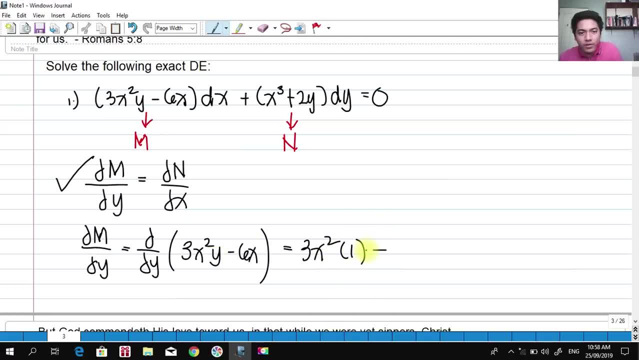 So this should be multiplied by 1.. Okay, Minus again. if we differentiate this, 6X, 6X, 6 is a constant multiplied by X, which is also a constant because we're differentiating it with respect to Y. 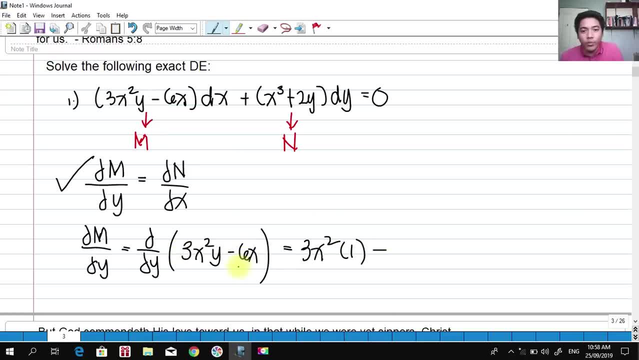 So this 6X is actually will become 0, because 6X is actually a constant. So what will happen? the partial derivative of M with respect to Y would now be 3X squared. Okay, I hope you get it. So the other one, we will try to get the partial derivative of M with respect to X, okay, 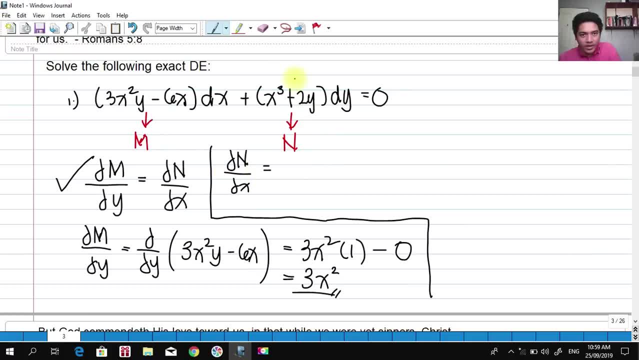 And that is equal to N as a function of X and Y. And here is our N. So our N is X cubed plus 2Y. So what will happen is that if we get the partial derivative of that, we will be having: 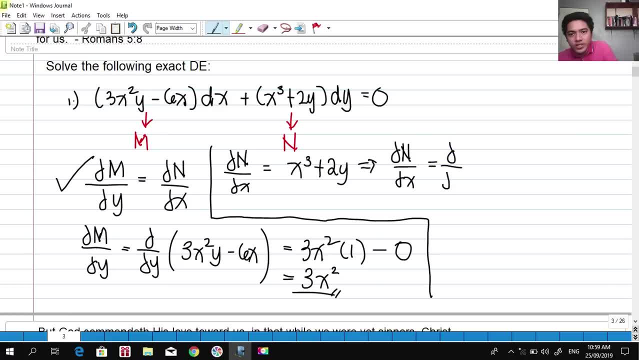 what This? The partial, with respect to X, of X cubed plus 2Y. okay, So what will happen? we are differentiating with respect to X, So any other variables other than X is considered as constant. So in this case, if we differentiate it with respect to X, this would be 3X squared plus. 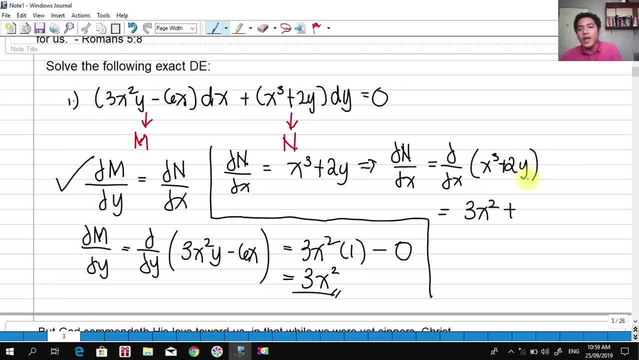 we have a constant, Okay, We have 2Y here, and any other variable again, except for X, is considered as constant. So the derivative of this 2 times Y, where Y is also a constant because we're differentiating with respect to X- that is equivalent to 0, because the derivative of a constant is 0. 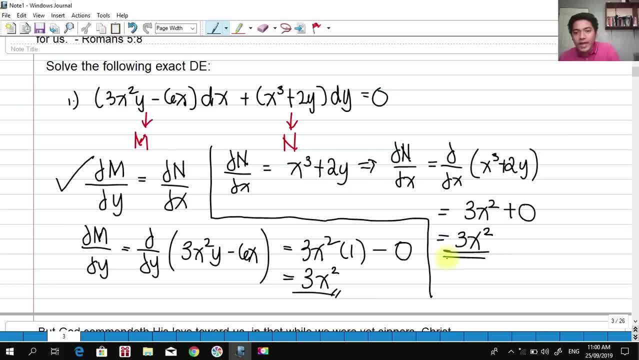 So what will happen? we have 3X squared also, hence, we have proven that this given DE is an exact differential equation. So hence, therefore, we can conclude that this is exact. okay, And now in order for us to solve the exact DE, because this is not the final answer. 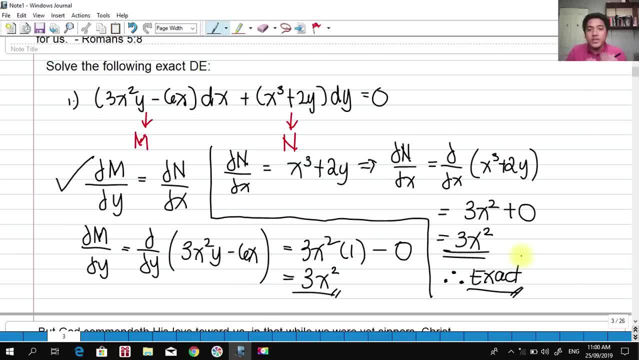 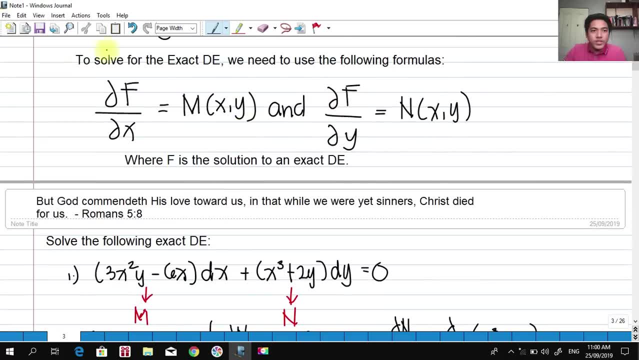 this is only a test for exactness of the DE, but this is not the final answer. In order for us to get the final answer, we shall be using our formula while ago, which is this: The partial derivative of M with respect to X is equal to M as a function of X and Y, and. 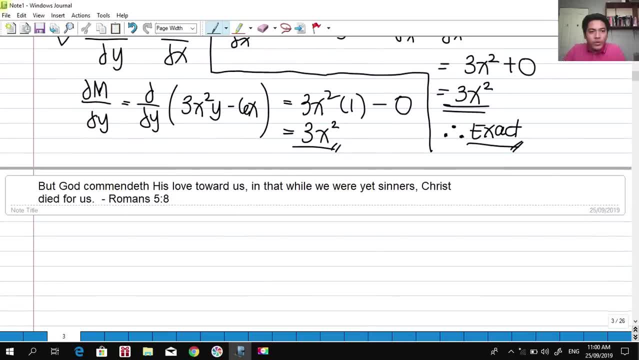 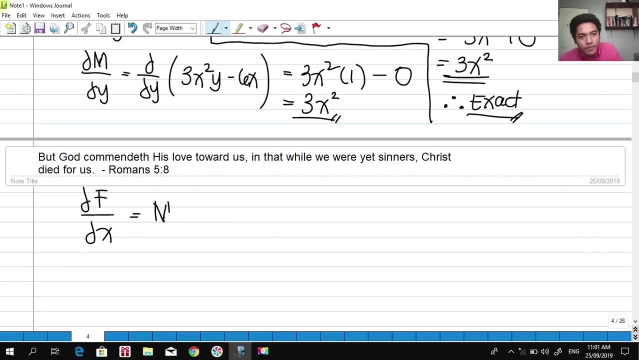 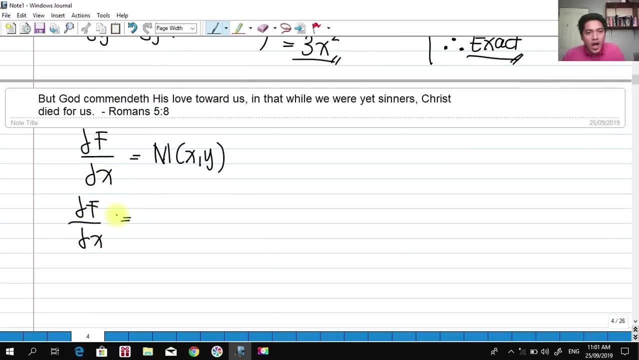 this formula also. So first we're going to solve: the partial derivative of M. F with respect to X is equal to the M as a function of X and Y. So what will happen here? we have the partial of F with respect to X, our M, again our M. 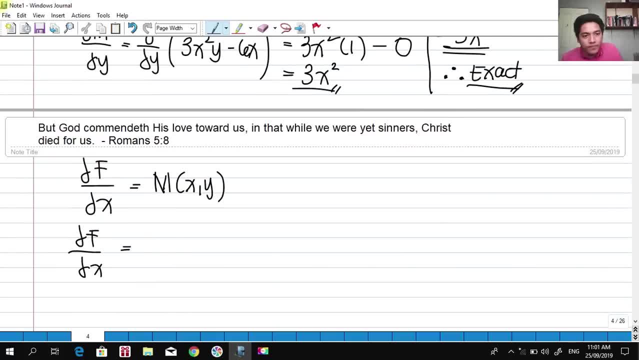 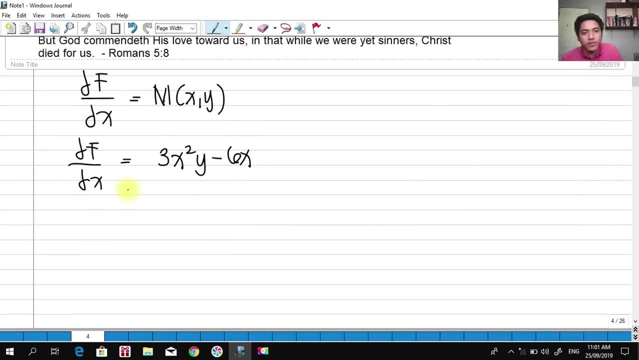 is 3X squared Y minus 6X. Okay, If I'm going to cross-multiply DX or partial of X with, on the other side of our equation, we have partial of F. okay, we have 3X squared Y minus 6X, partial of X, all right. 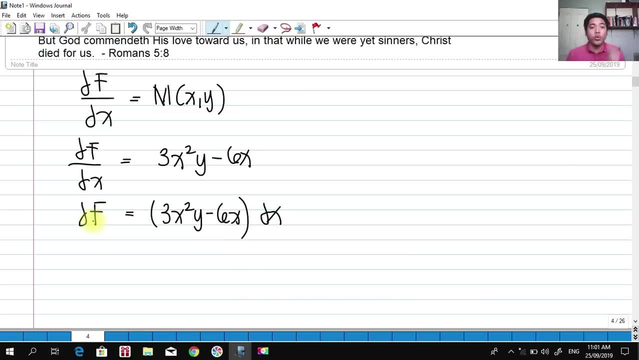 And we say class, that F is the solution to our differential equation. This is partial of F. So if I'm going to integrate both of these equations, I'm going to integrate both of the sides of our equation. I shall be getting F here, which is this: F is the solution to 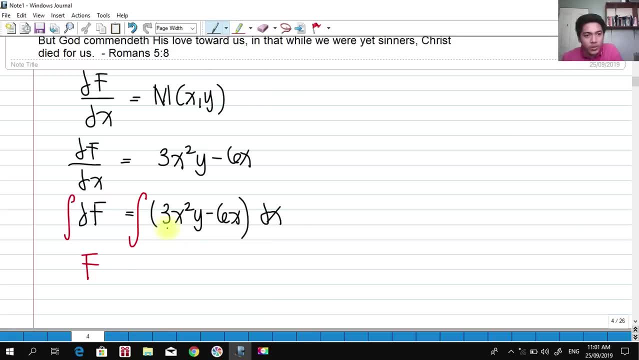 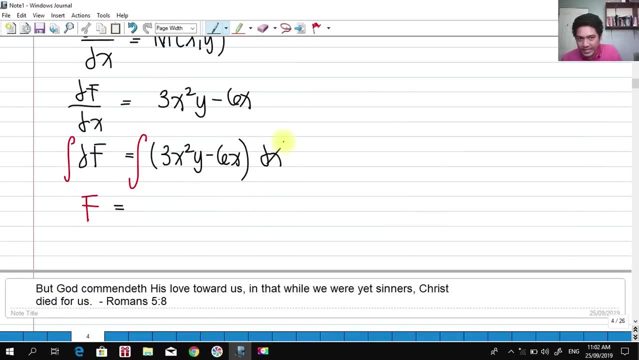 our differential equation. So what will happen? This should be equal to now. how do we integrate this? This is with respect to DX. okay, So partial of X, So we can actually what By properties of integral we have, we can distribute the integral sign on this, because 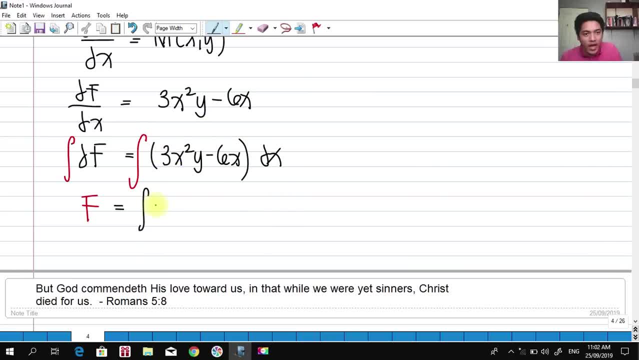 this is a differential, Okay, And also the presence of DX. So we have 3X squared Y. DX, or partial of X is still okay, minus the integral of 6X, partial of X or simply DX, okay. So what are we going to do? 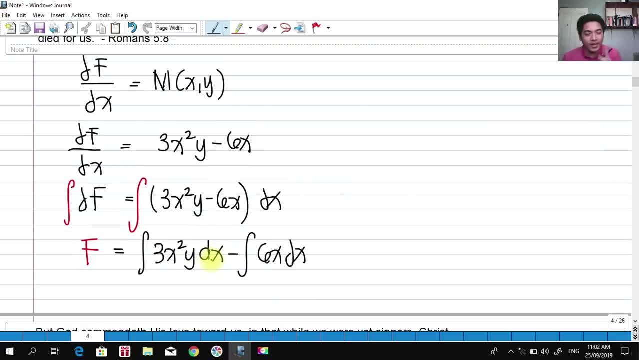 Okay, We are differentiating or integrating, I'm sorry. we are integrating in terms of X, So any other variable rather than X okay, Should be X Okay. So what will happen here? We are going to have this: Y is treated as constant. 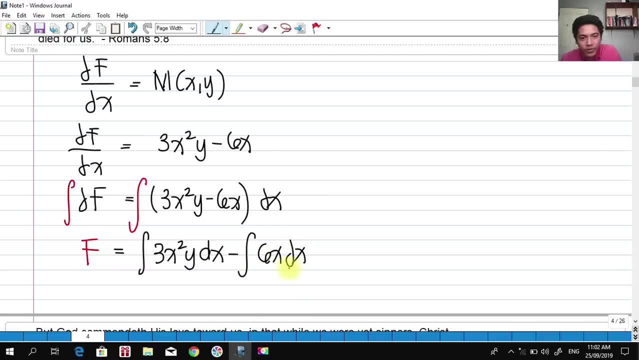 So this Y is treated as constant and we have no constants here, but the six, okay, And also the three here. So what can happen here is that it should now be equal to. I can factor out the constant three and Y inside, outside of the integral, so we have three Y integral of X squared. 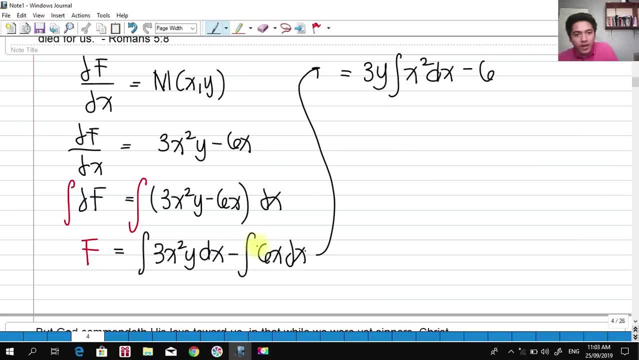 DX minus six. I can factor out six because that is a constant. Okay, Yeah, x dx, so integrate. so we have 3y x cubed over 3. that's the integral of x squared minus 6 times x squared over 2. okay, plus, of course, when we do integral, we have a. 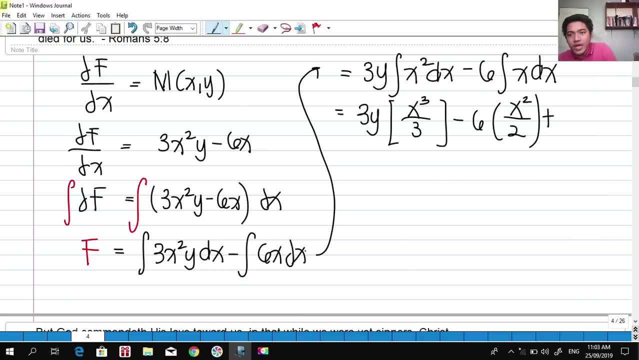 constant. but here the constant is actually what is in terms of Q of Y. I will explain later after. we simplify this: y, Q of Y. okay, so we can see that this will cancel. 6 over 2 is simply 3, so we have now x cube of y, x cube y minus. 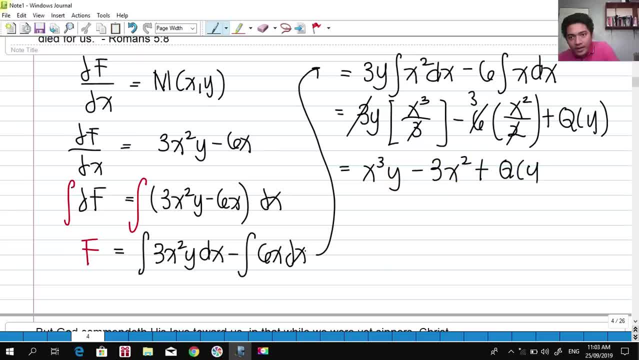 3x squared plus and a constant Q in terms of y, y, Q of y. why not simply see: no, no, also that this is plus C. this can be also plus C, but more than that, this is a constant. so we can see that this is a constant, so. 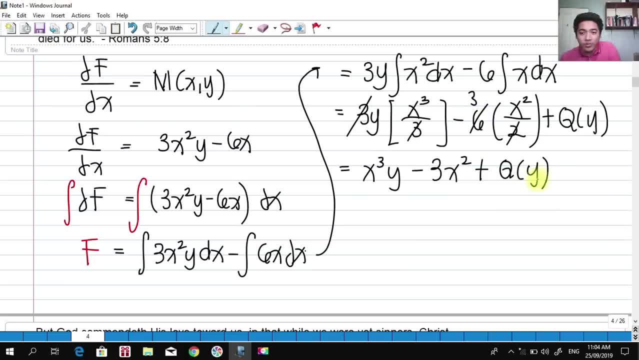 specifically, this is Q of Y as a function of Y. why? because we know that this is now the F. okay, this is now the F. the whole function is there and our original given is this partial of F with respect to X. so, if I'm going to 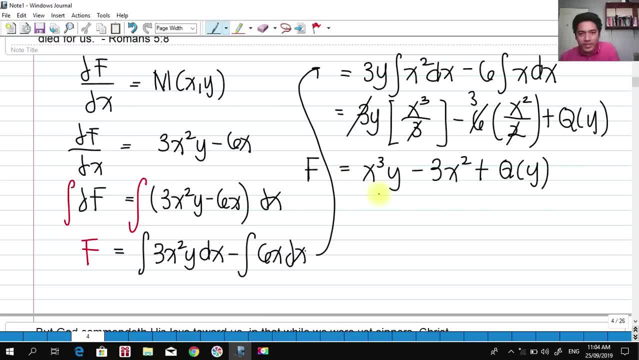 differentiate this with respect to X. I shall be arriving at this, okay, because that is, that is the opposite of integration, the differential derivative, right. so even if I'm going to add, let's say, Q of Y, even if I'm going to add y here, let's say Q of y is equal to. 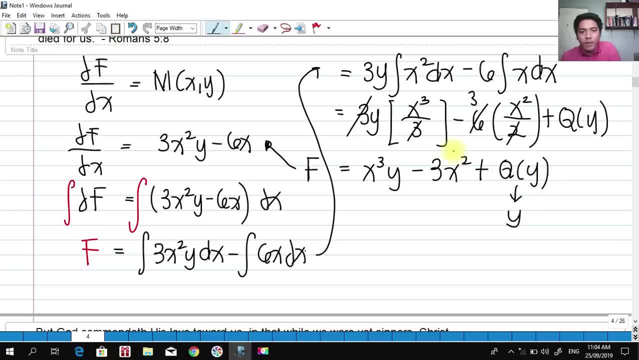 Y and I'm going to get the partial derivative, partial derivative of this F with respect to X. okay, I shall be still arriving at this answer. why? because if I'm going to get the partial derivative, this F with respect to x, I should be still arriving- and that's the ABC- me into that to the. I discovered it should be up here and immediately bring it down to the radical derivative with respect to X. what, let's say, I shouldнов contribute my derivative to myself will possibly better or do even greater, or be like that, the less gonna be higher than féleigh minus the partial derivative d, Denver classiries, which will be ducked down there and there will become a minus 2 to your currentoral derivative. and keep myself out prior to perhaps…. 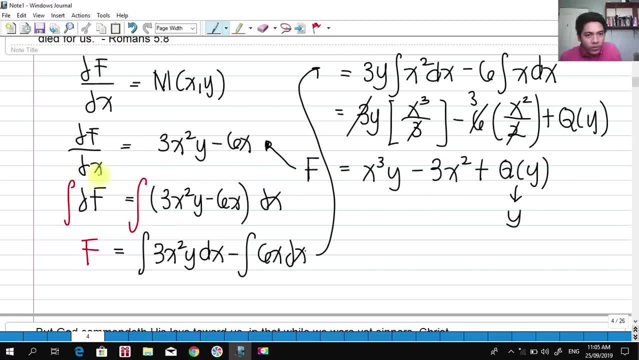 then I'm going to say, not only for the slowข: when you write this formula- and let me kick one- get the partial derivative of this f with respect to x, even if i have a y term here, okay, the result would always be this: because y here is treated as constant, and i hope you get it so. okay, so we have. 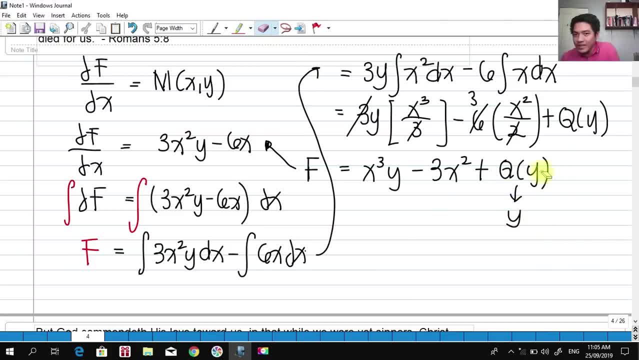 this q of y here? okay, so, because if we again, if we differentiate it with respect to partial of x, this would be still zero. okay, so this is a constant, but in terms of y, because we are partially differentiating it with respect to x, and i hope that's clear. so, because this q of y 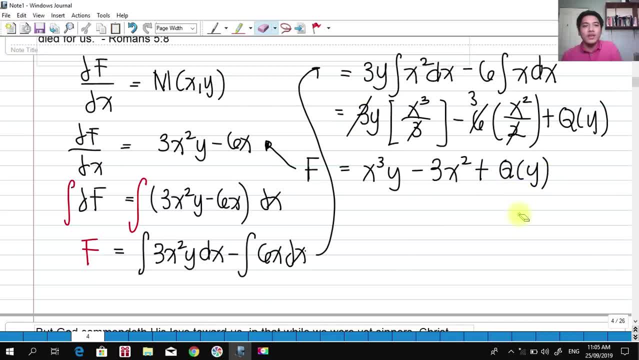 is important, so let me just erase this. i hope you got it, okay. so again, is this now the answer? yes, we can use this as our answer, but we don't know the value of q of y, so what are we going to do? is so? we are not yet. 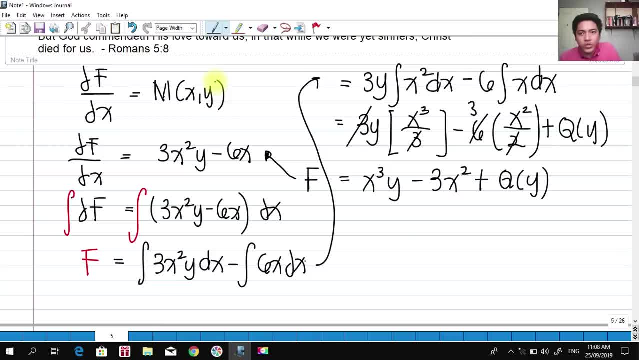 done in our solution. let's take note that we only get the partial of f with respect to x. but how about the partial of x? partial derivative of f with respect to y is equal to the n as a function of x- y, because that is our formula, that is our second formula, and if you get this, 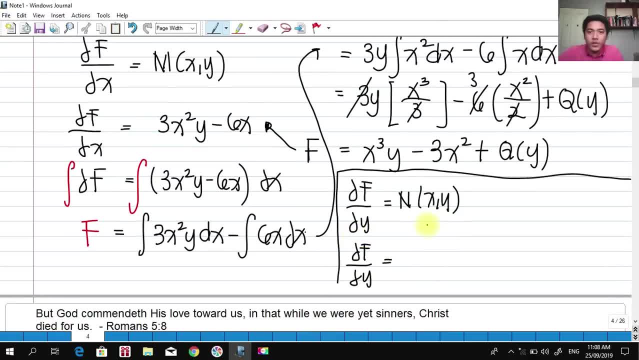 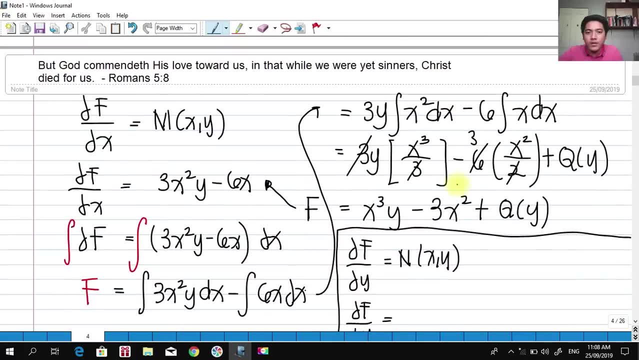 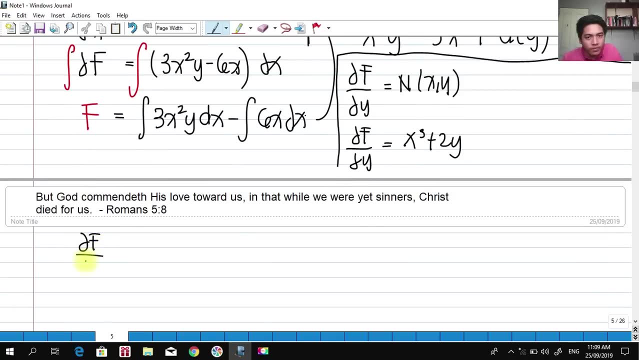 partial of f with respect to y is equal. what is n in terms of x- y? that is x cube plus 2y, x plus 2y here. so we have x cube plus 2y and if we're going to cross, multiply that partial of f. 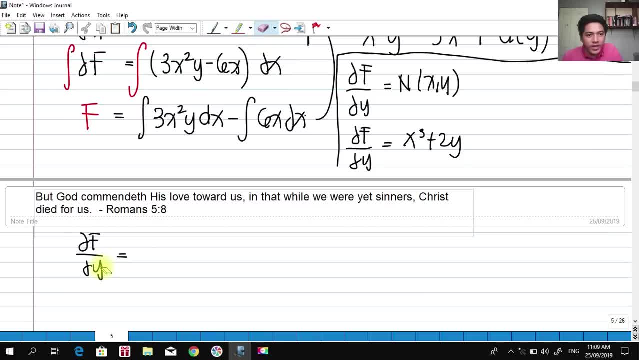 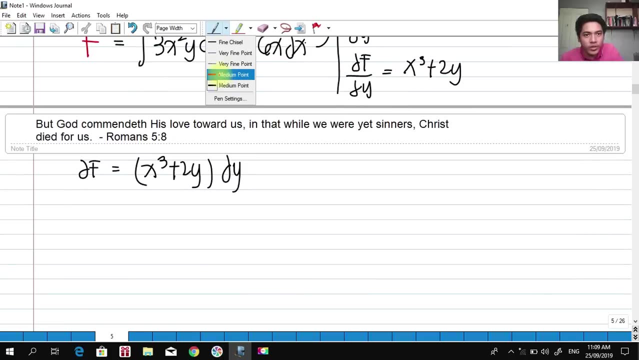 with respect to y: okay, uh, cross multiplication- okay, so we have now partial of f- is equal now to x cube plus 2y. okay, dy here and we are after the f. so we're going to integrate both sides to get the solution of x and y, and we're going to integrate both sides to get the solution of x and y. 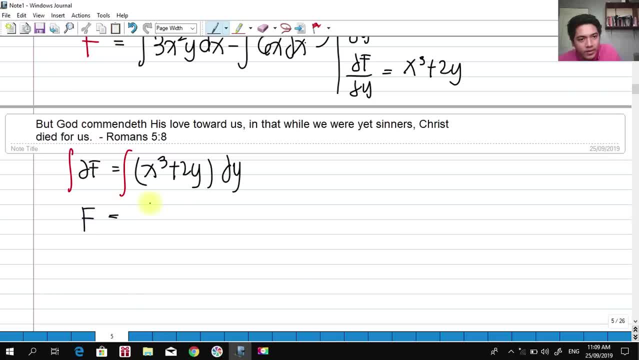 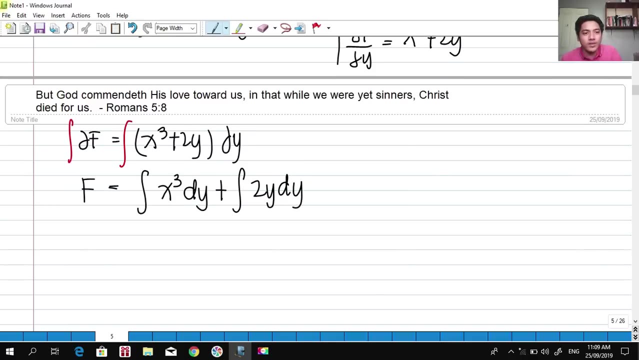 so we have: f is equal to the integral of x cube dy plus the integral of 2y dy. notice here that we are integrating in terms of y, so any other variables, okay, other than y, is considered as constant. so in this case i can factor out outside of the integral this: x cube dy and: 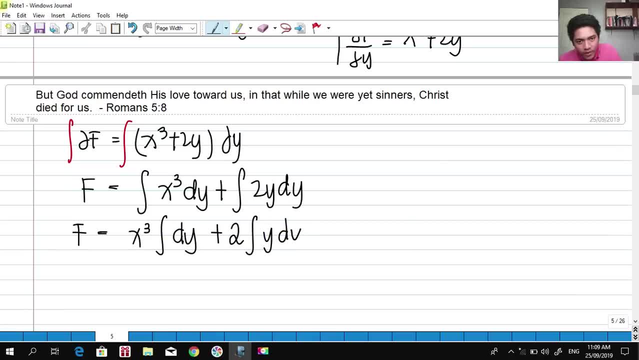 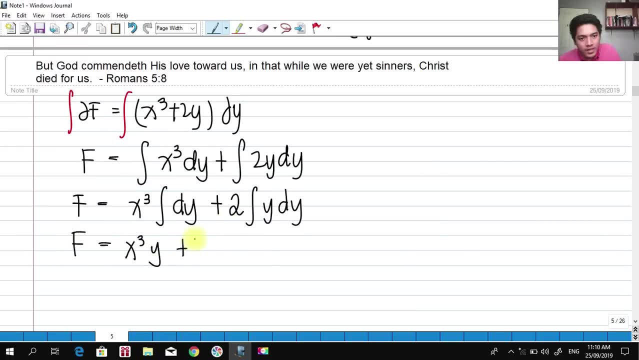 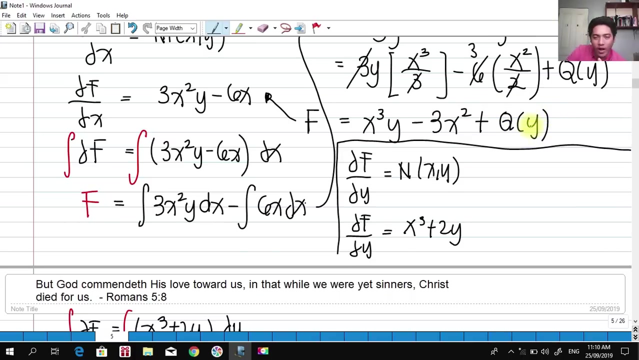 i can factor out to the integral of y dy, so we're going to get that. we shall be having x cube of y plus 2y squared over 2. okay, this should be cancelled. and plus, okay, if we have a q of y here, which is a term that is purely in terms of y. 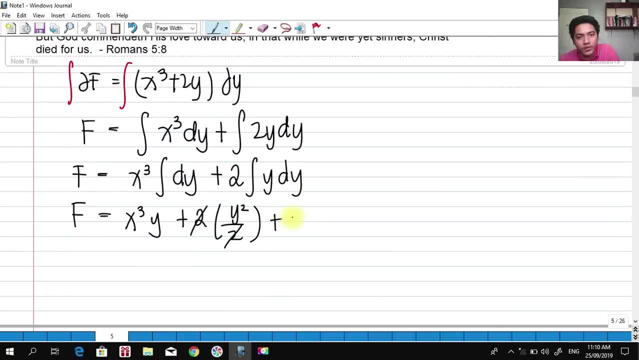 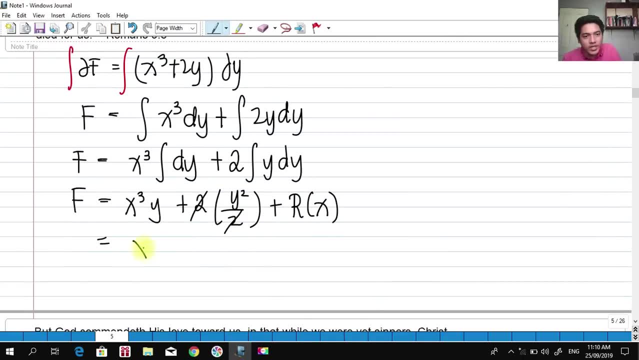 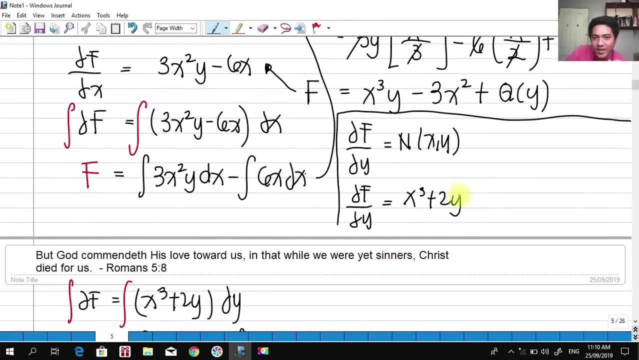 so we shall be having also another term here, a constant r of x. okay, because, again okay, i'm going to differentiate this plus r of x, because, again okay, if i'm going to differentiate this with respect to y, even if i have a term x here, pure terms in x, the result will always be this: okay, okay, so even. 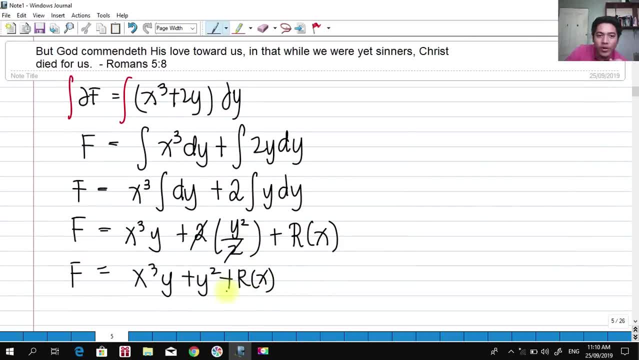 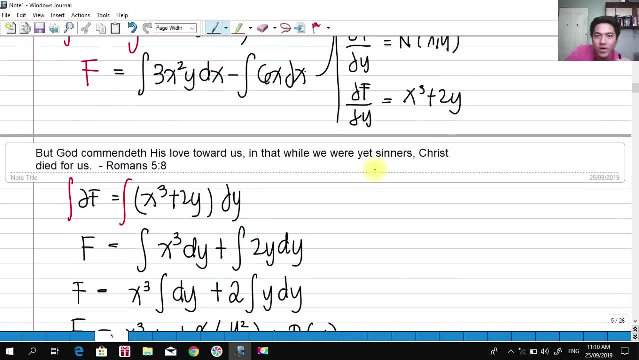 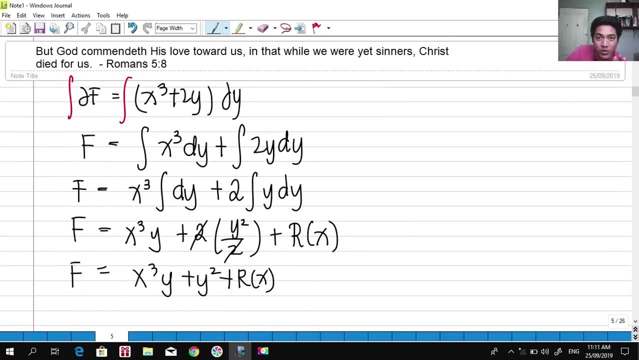 if i have an x term here, okay, if i'm going to partially differentiate it with respect to y, this is treated as constant, okay? so i will be still arriving at this answer. it's morely, merely more of a constant, but it is in terms of x, because we're doing a partial derivative. 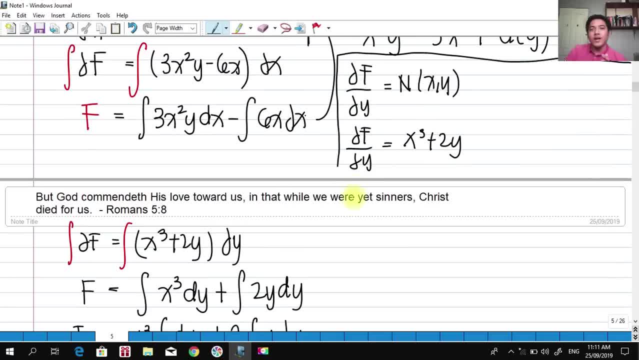 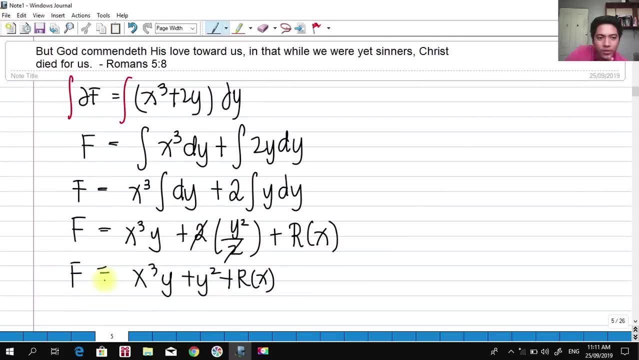 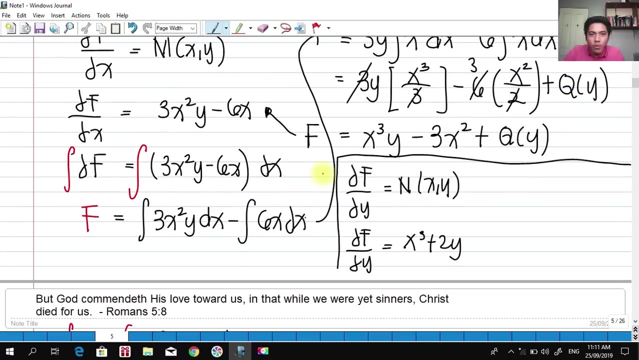 okay. so, sir, what is the final answer? so we need to determine the q of y and the r of x. so here we have: f is equals to x cube y plus y, squared plus r of x. and here we have x cube of y minus t x squared plus q of y. notice that they are both equal to f. so if i'm going to equate, 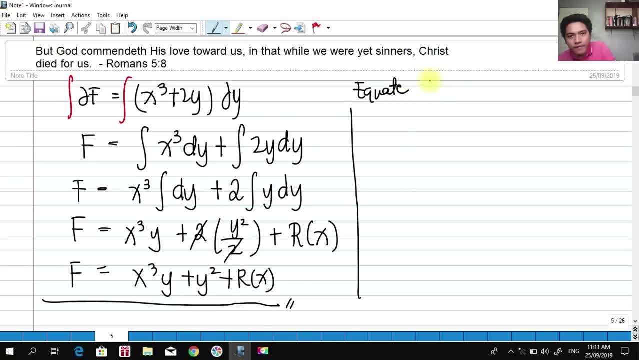 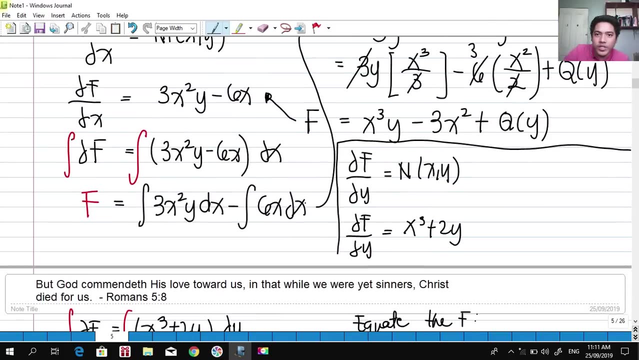 okay, equate the f. okay, the f, the two f's. okay, so we have. first we have this: let's say: x, x cubed y plus y, squared plus r of x, is equal to the other f here, which is x cubed y, x. 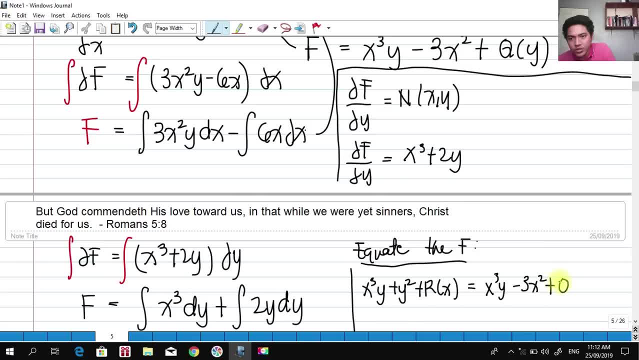 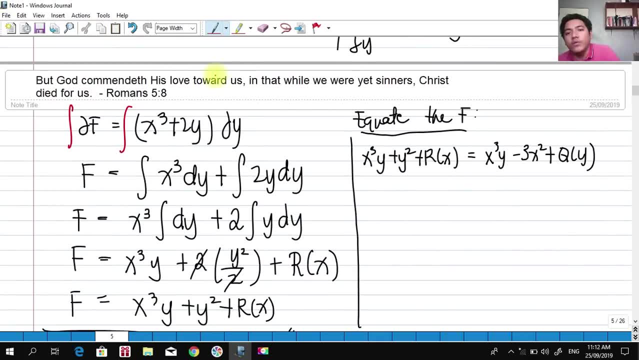 cubed y minus 3x, squared plus q of y: okay, so we're going to find the values of f of x and q of y. as you can see. x cubed y would cancel. okay, x cubed y would cancel. and. 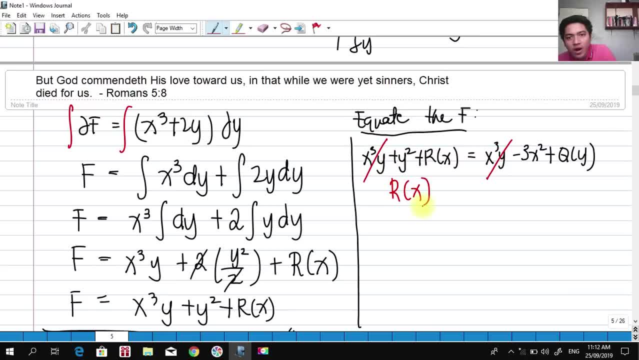 by inspection, our value of r of x on the other side is negative 3x squared. why? because r of x is purely in terms of x and we have a term here on the other side that is purely in terms of x, which is negative 3x squared. hence r of x is equal to negative 3x squared. 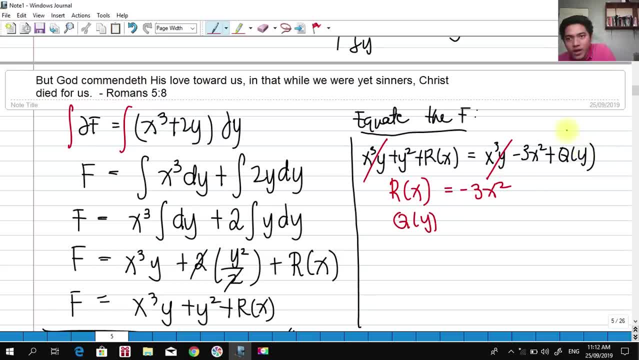 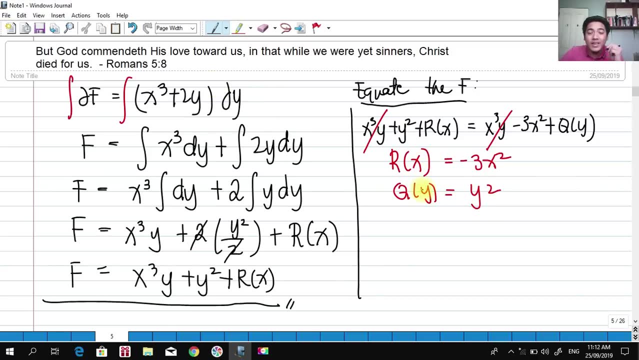 how about q of y? here is our q of y, and on the other side of the equation, we have a purely in terms of y. Okay, so, upon okay, upon determining r of x and q of y, we shall be getting the answer. 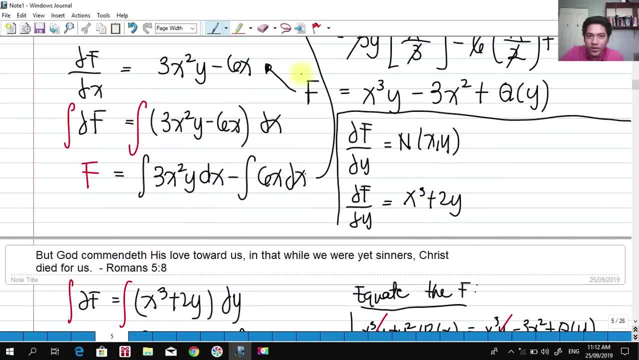 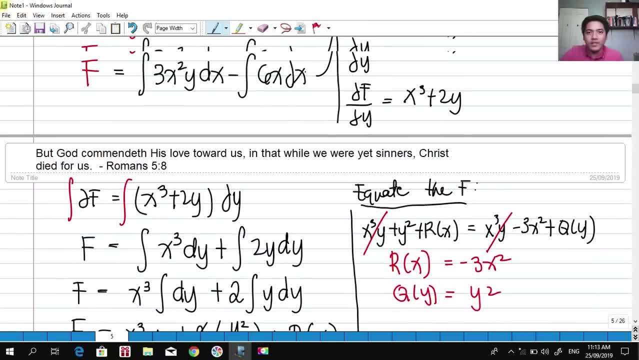 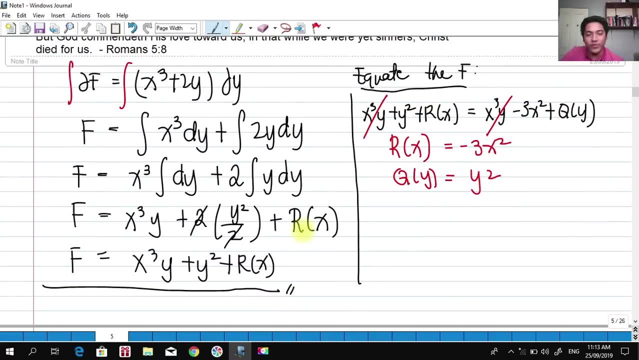 by simply substituting the value of q of y, here in our first f function, or the r of x, here in our second f function. only that this f, okay, this function f will be replaced by a constant c. okay, because whenever we do integration, we are having a constant c. 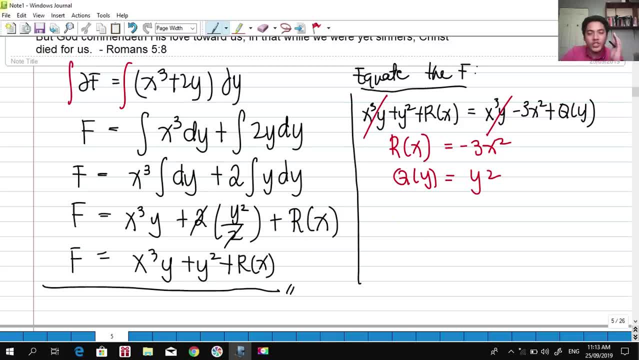 which is a very common or a general constant c. so if I'm going to use this, I will be having x cubed y. the general solution for our d is x cubed y plus y squared plus. what is this? r of x. okay, that will become negative, because this is negative. 3x cubed. 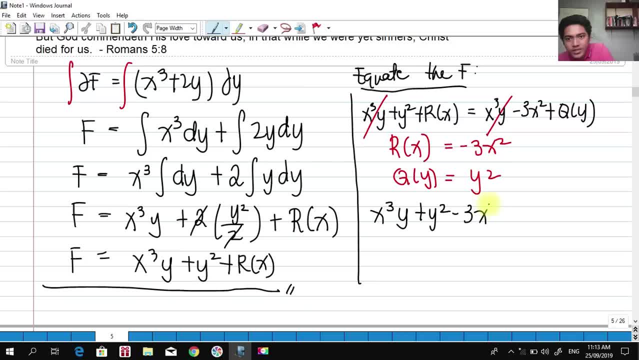 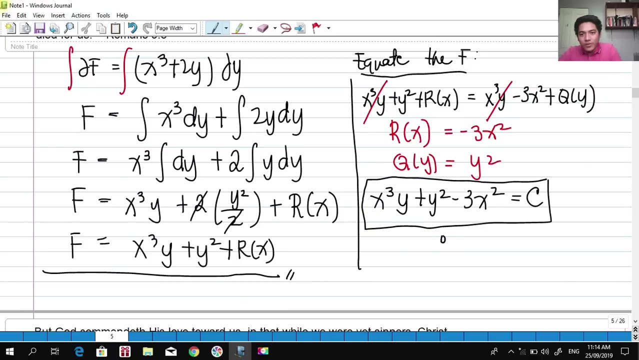 so that would become negative 3x squared, okay, Okay, Okay, Okay, jego is equal to f, which is equal to c, and this should be now our general equation. Okay, Sir, Can we use also this? Okay, if you use this, No problem. if you use the other one, the other f here, no problem. 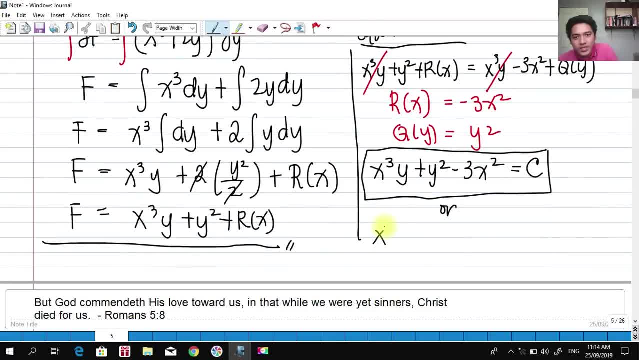 we have x cubed y minus 3 x squared. So x cubed y minus 3 x squared plus the Q of Y, which is plus Y squared, and the other side of the equation, the F, will now become the C. so in other words, even if you use the first F as a, 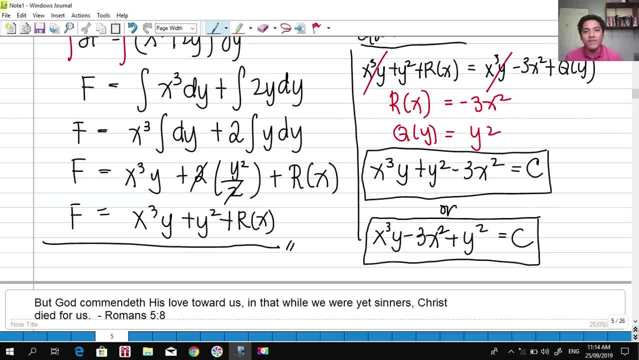 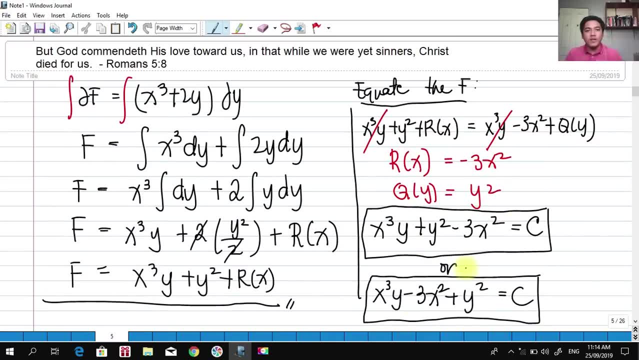 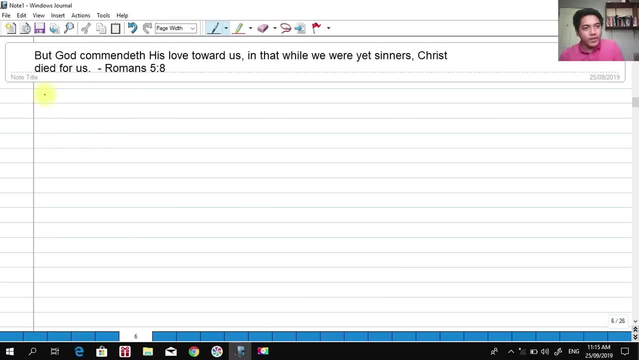 solution or second F as a solution, you will still be arriving at the same answer, and hence this should be our answer for the exact DE given in the problem. okay, let's try to solve again another problem. for problem number two, we have 2x cubed minus X Y squared minus 2y plus 3 DX minus X squared Y plus 2x. 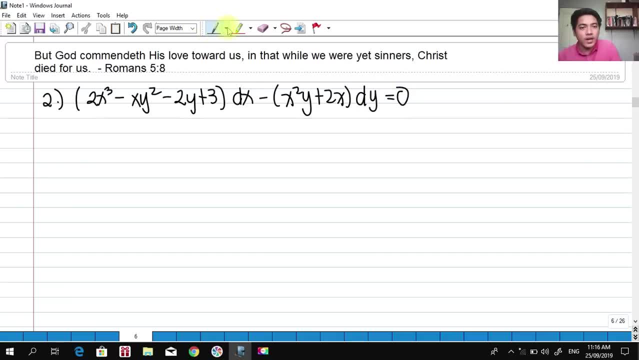 DY is equals to 0. notice again that this is a problem that we have to solve. in order to solve this problem, we have to solve this problem. we have to solve this problem. we have to solve this problem. this should be our M. okay, and this should be our M. so, upon performing test. 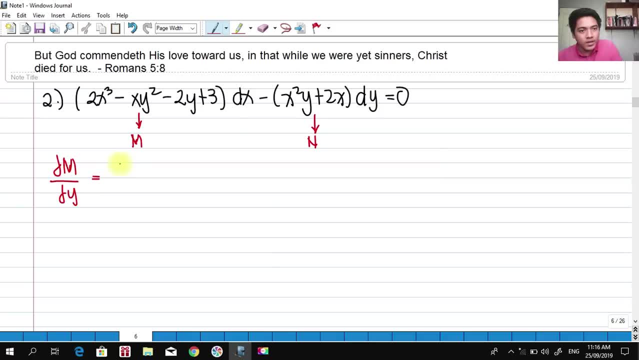 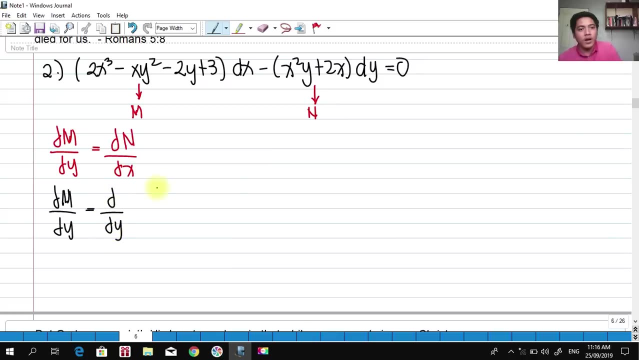 of exactness, partial of M with respect to Y. that should be equal to partial of N with respect to X. so, upon performing that, we shall perform that. okay. partial of M with respect to Y. okay, so this should be the partial of the function M with respect to Y, which is 2x cubed minus X. 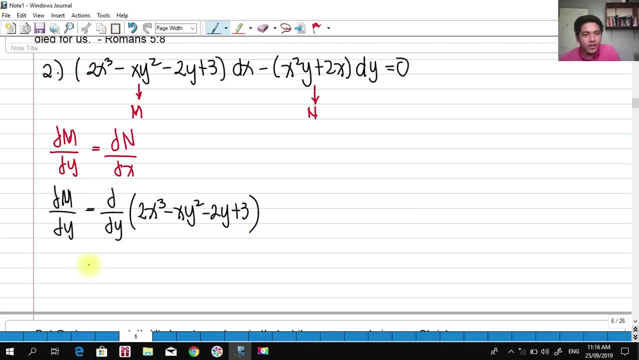 Y squared minus 2y plus 3. okay, so, as you can see here, this term does not have any Y terms in it. so any other variable except for Y is considered as a constant. so the derivative of this constant is 0, 2x cubed the derivative. 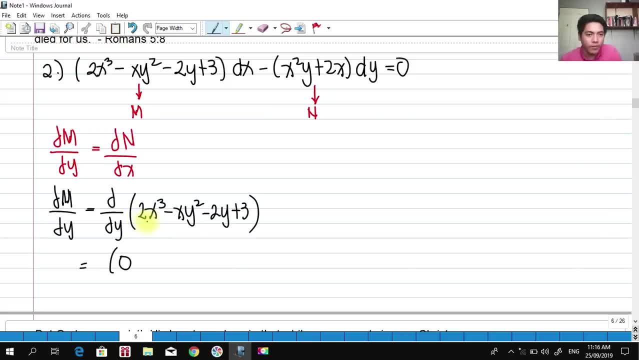 of partial derivative of what's 2x, cubed with respect to Y is 0. how about this? alright. with respect to Y, that is 2y. okay, so now we have to do something here. Okay, but since x is considered as constant, that should be 2xy. 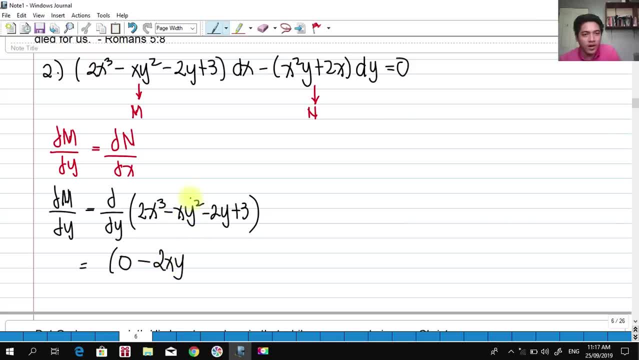 Okay, so this should be considered as constant. You try to differentiate this. And this term, okay with respect to y, is minus 2.. And this term with respect to y, that is a constant plus 0.. So hence our partial derivative of m with respect to y is negative: 2xy minus 2.. 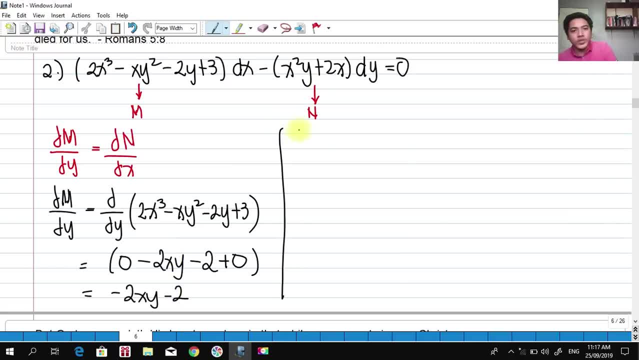 Okay, and we shall get the partial of n with respect to x. Okay, that is, of course, this is a negative sign. So if I'm going to distribute the negative sign, you must do that. Negative x squared y minus 2x. 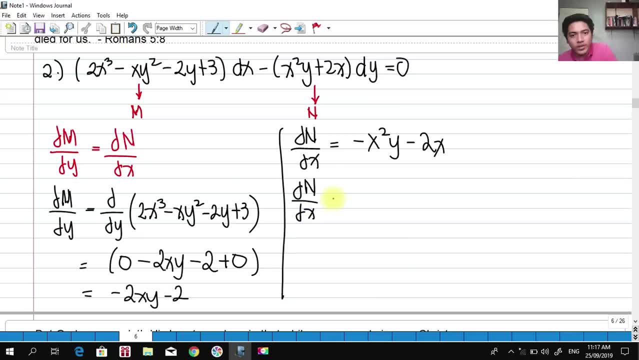 Okay, so if I'm going to differentiate that with respect to x, okay, this function of n, So any other variables aside from x, is considered as constant. So get the derivative of this negative x squared y with respect. partial derivative with respect to x. 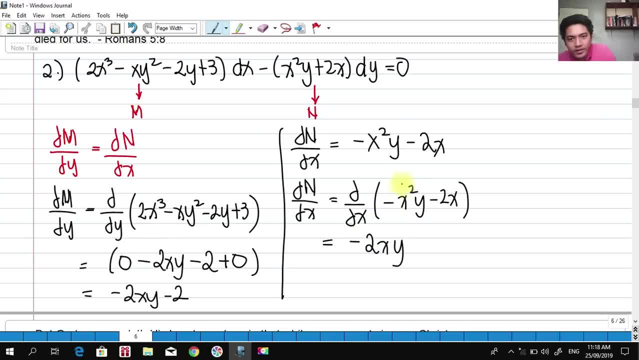 So that is negative 2xy. Okay, and partial derivative of this, with respect to x, that is minus 2.. Hence negative 2xy minus 2, negative 2xy minus 2.. Therefore we have negative 2xy minus 2.. 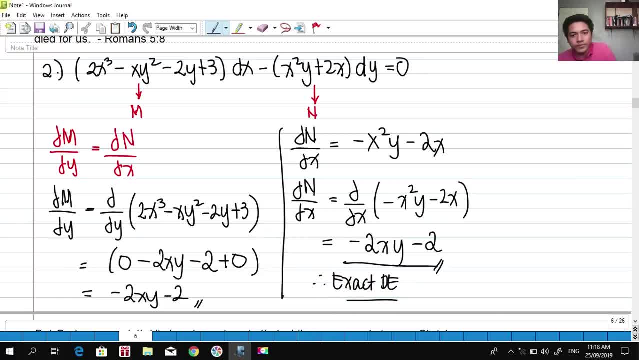 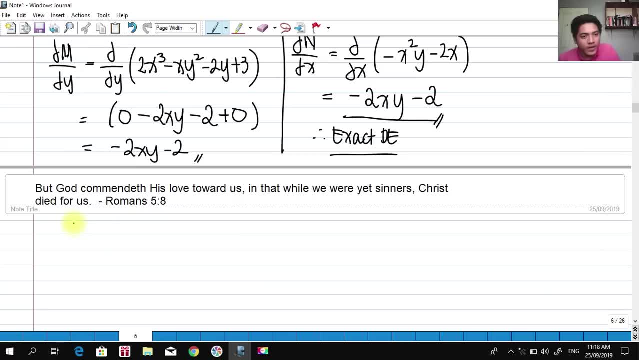 So we have an exact D And again we shall be solving the exact solution, or the solution for this D, by performing again the partial of m, okay, with respect to x, And that is equal. okay, not partial of m, but partial of the function f. 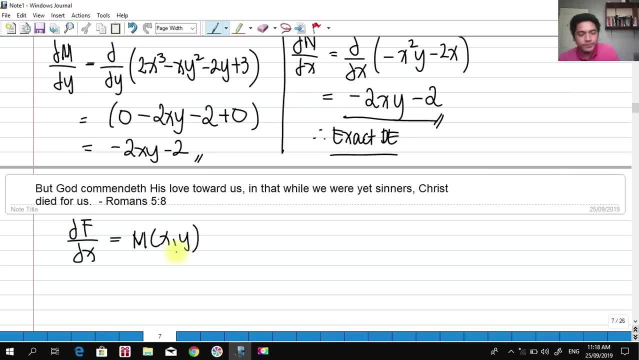 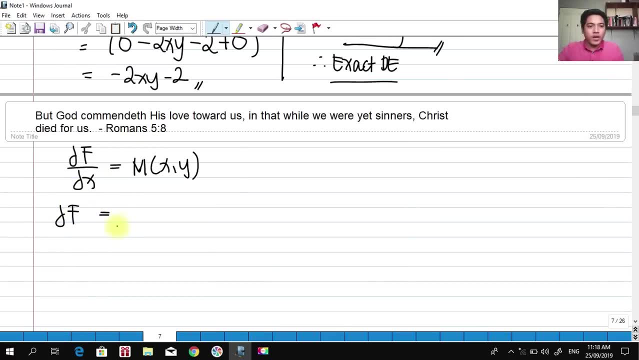 And now equal to the m as function of xy. Okay, so again, if I'm going to cross multiply this, this should be partial of f. okay, multiplied by m, what is our m 2x cubed minus xy squared? 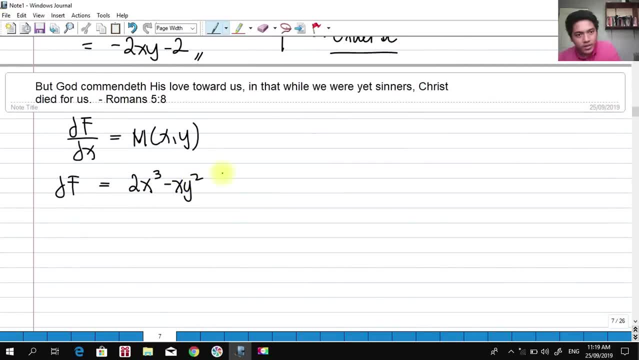 So we have 2x cubed minus xy squared, minus 2y plus 3.. Okay, so cross multiplying this, we have now dx here. So if I'm going to integrate both sides so as to get the f, okay, because that is our solution again. 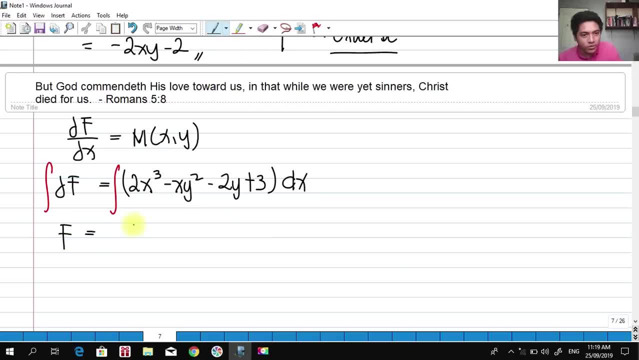 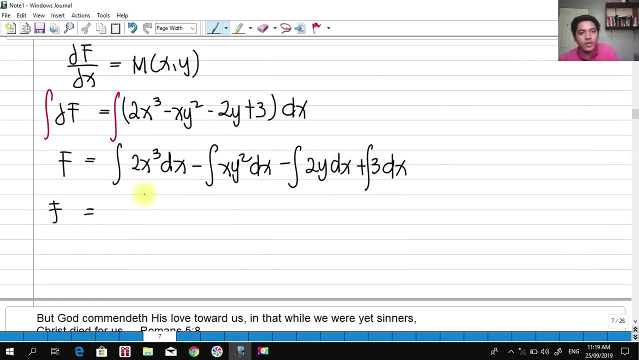 So I have here: f is equal Now 2, distributing the integral in the dx side, we have 2x cubed dx minus xy squared dx, minus the integral of 2ydx, plus the integral of 3dx. So, and again we are integrating with respect to x. 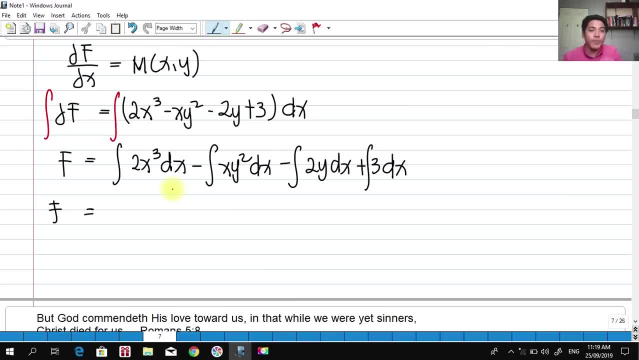 So any other variable aside from x is considered as constant. So we have- I can factor out: 2. Outside of the integral side we have x cubed dx. here I can factor out y squared here, because we are integrating with respect to x. 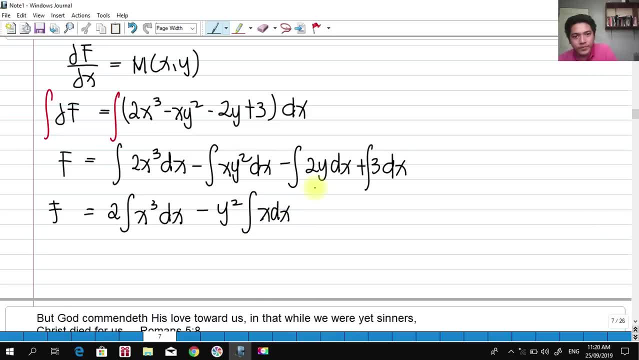 So y squared integral of x, dx. I can factor out 2 and y here: 2y, because we are integrating with respect to dx minus 2y integral of dx. I can factor out 3 here: 3. integral of dx. 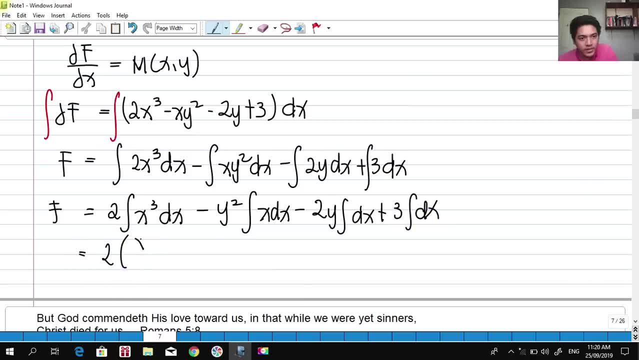 So in integrate. so we have 2x raised to 4 over 4, okay, minus y. squared x, squared over 2, minus 2y, the integral of dx is simply x plus 3 times the integral of dx is simply x. 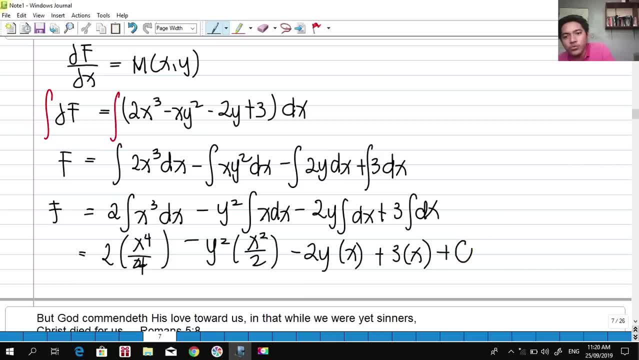 And of course, plus Q of y. okay, Don't forget the Q of y. And again, we can simplify: 2 over 4 is 1 half, So, yeah, So we don't have any other to simplify, So let's rewrite that: 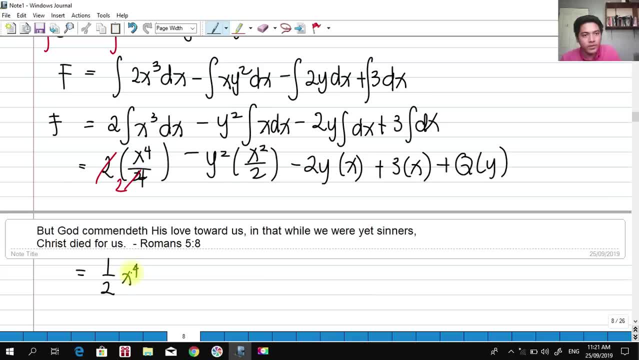 So we have 1 half x raised to 4, minus 1 half x squared y squared okay. x squared y squared over 2, minus 2xy plus 3x, plus Q of y, And that is our first f. 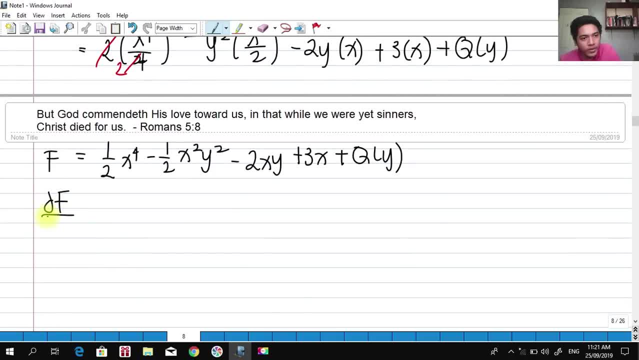 How about the second f? So partial of f With respect to y is equals to the n in terms of xy. So partial of f? n of xy is- don't forget the negative, negative x squared y minus 2x. 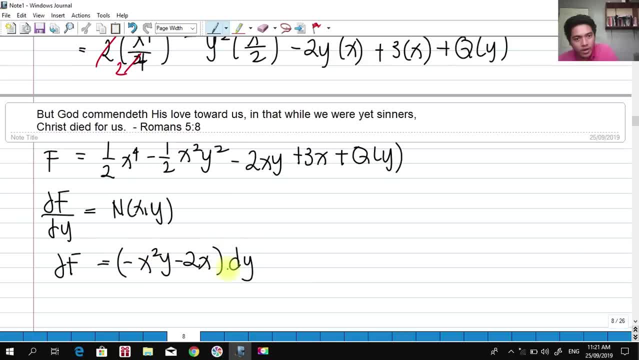 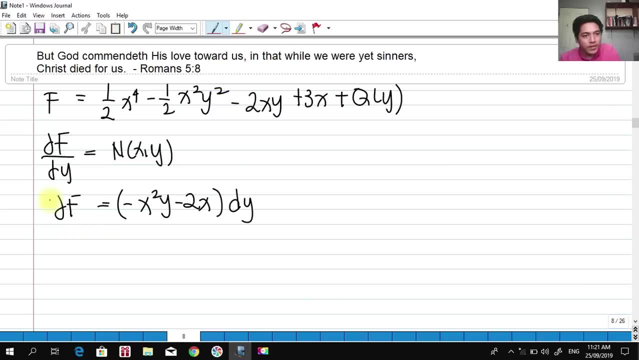 And of course this is multiplied by dy, because I cross, multiply dy here. So if I'm going to get again the integral of both sides of our equation, we shall. We'll be getting. f is equals to integral of negative x squared y dy minus integral of 2x dy. 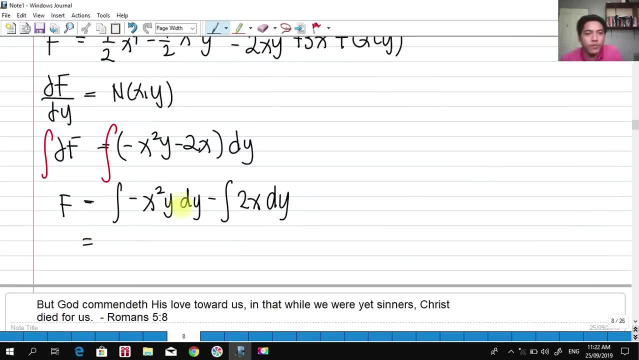 So any other variables aside from y is considered as constant because we're integrating again with respect to y. So we have negative x squared integral of y, dy minus. I can factor out 2x here because we're integrating with respect to. 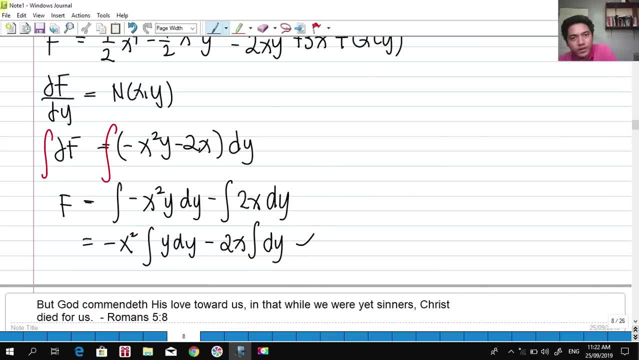 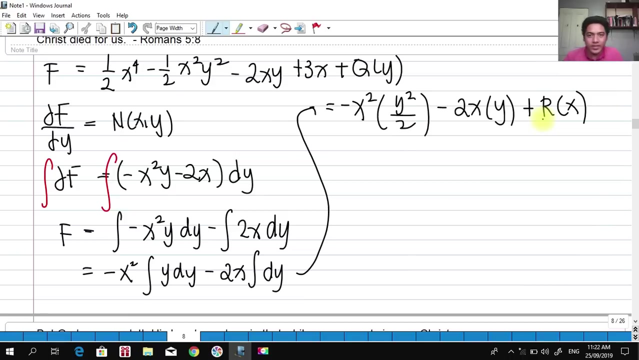 So what will happen? we have negative x squared y squared over 2, okay, minus 2x. integral of dy is y. okay, plus R of x. Okay, don't forget that. A constant in purely in terms of x. 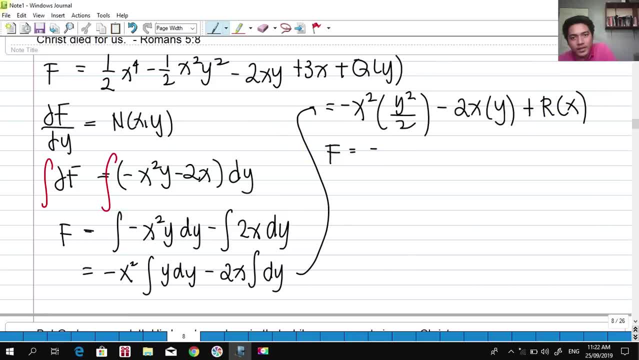 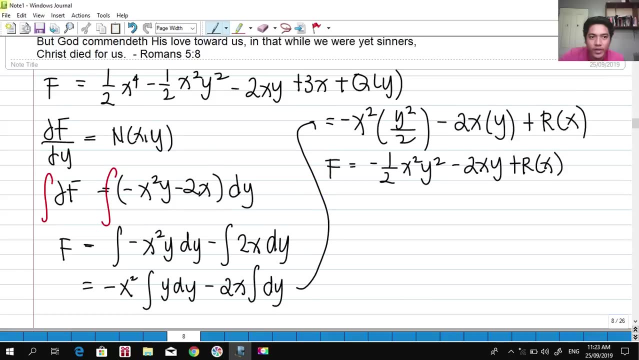 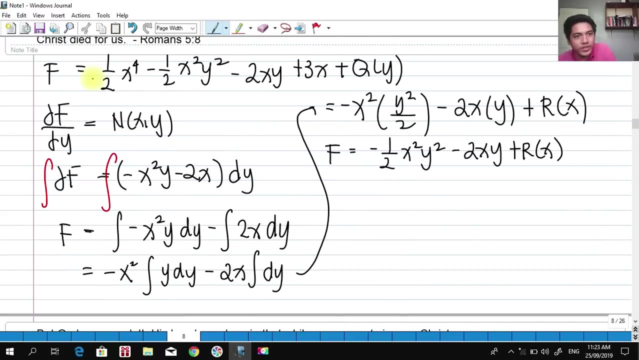 So we have now f as negative, 1 half x squared, y squared minus 2xy plus R of x, And the last step is actually to determine the value of R of x and the Q of x. So if we are to equate the two, okay, wait, we should equate first this. 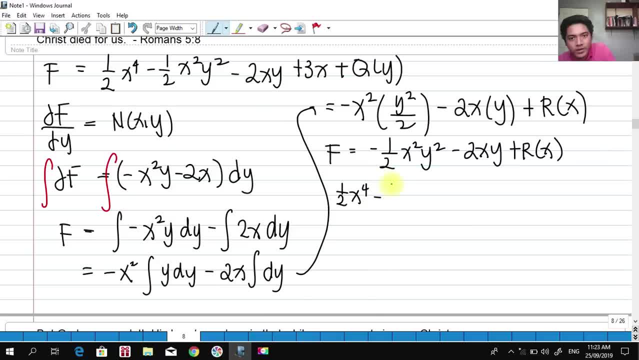 We have 1 half x raised to 4 minus 1 half x squared y squared minus 2xy plus 3x plus 2x. So we have 2x plus Q of y is now equal to negative: 1 half x squared y squared minus 2xy plus R of x. 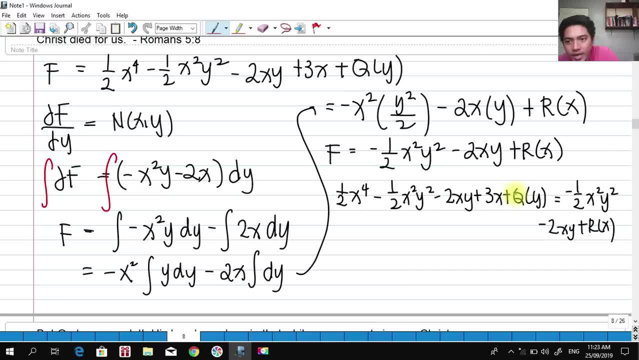 Okay. so, as you can see, upon simplifying, we can cancel out some terms. So we have negative 1 half x squared, y squared. We have negative 1 half x squared, y squared here. Okay, so we can also cancel out negative 2xy and negative 2xy here. 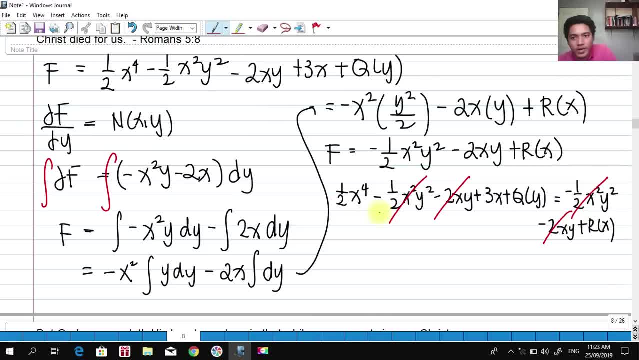 Okay, so We shall be determining what is the value, or we shall determine what's the value of Q of y. Okay, so Q of y as a function of y. on the other side of the equation there is none. Okay, so that is 0.. 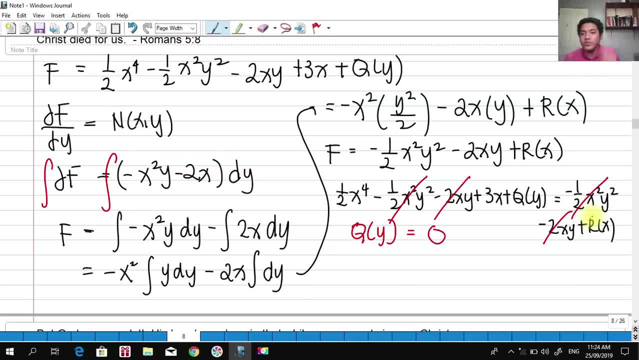 Because there is no other term here that is purely in terms of y on the other side of the equation, That definitely that is equal to 0. And R of x is now equal to the x term, Purely, purely expressing terms of x on the other side of the equation. 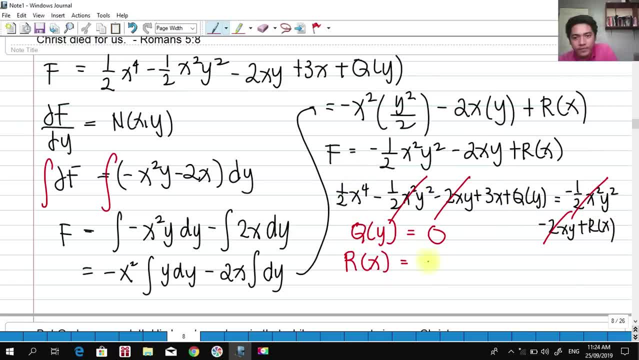 So we have R of x. on the other side of the equation, We have 1 half purely in terms of x, 1 half x raised to 4, plus here we have 3x, And hence we can use this one or this one to obtain our general solution for this exact D.